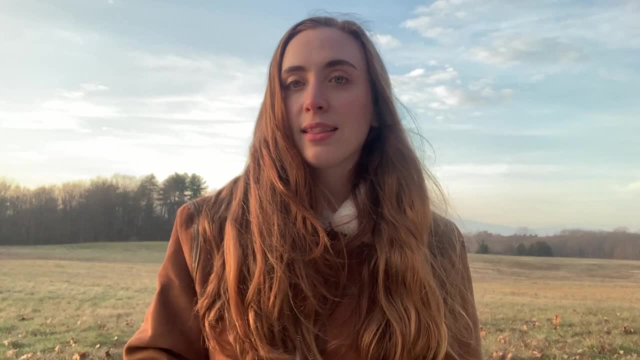 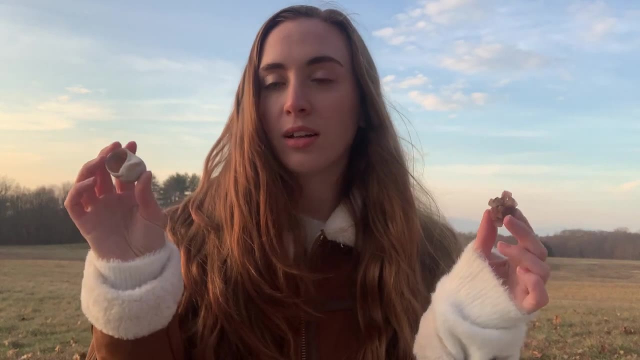 in geology is that they are inorganic. This means that they are not made from living materials or something that used to be living. For example, we have aragonite and a seashell. These are made out of the same elements. They have the same chemical properties. They have the same chemical properties. 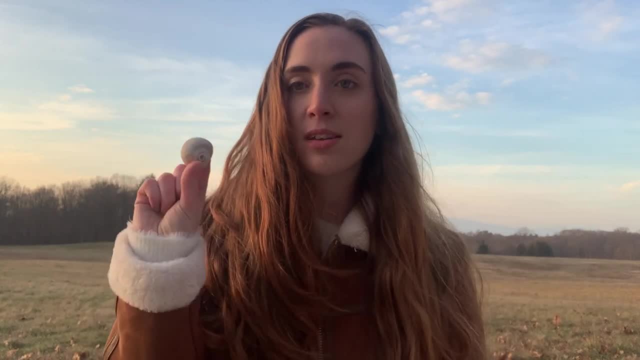 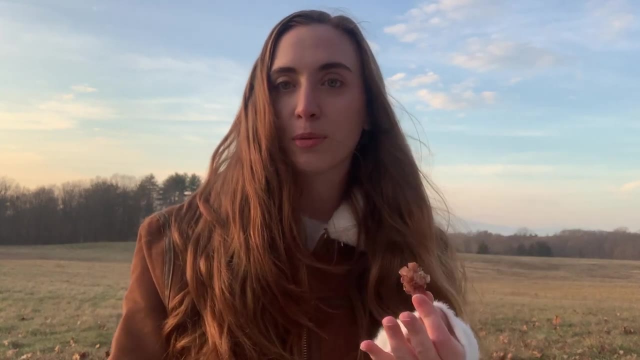 They have the same chemical formula but they are not both minerals. A seashell is not a mineral because it was made from a living organism, and aragonite was not made from a living organism. It was made from geological processes. The third characteristic of a mineral is that it must be. 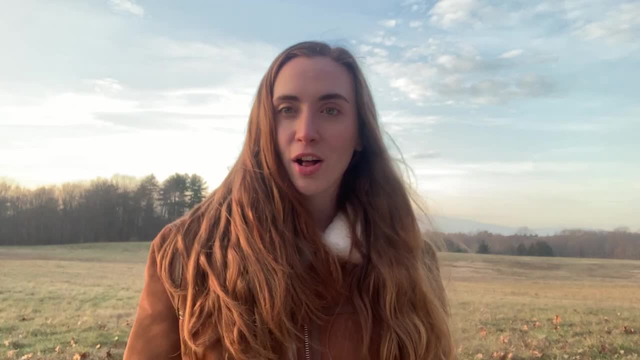 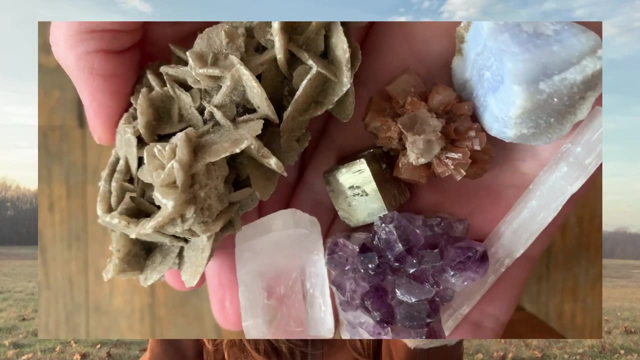 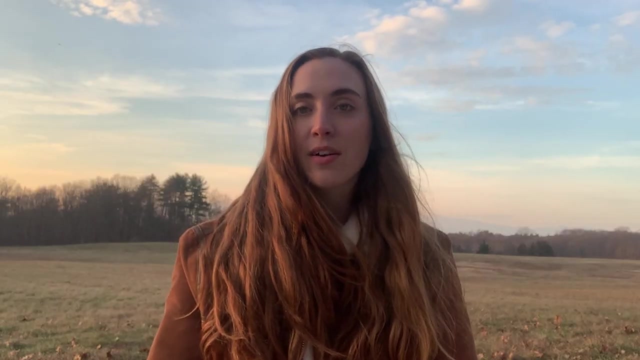 solid. This means that the mineral must be in a solid phase state at standard temperature and pressure. So right now these are solid. Mercury, for example, is not a mineral because it is liquid at room temperature. The fourth characteristic of all minerals is that they have to have a 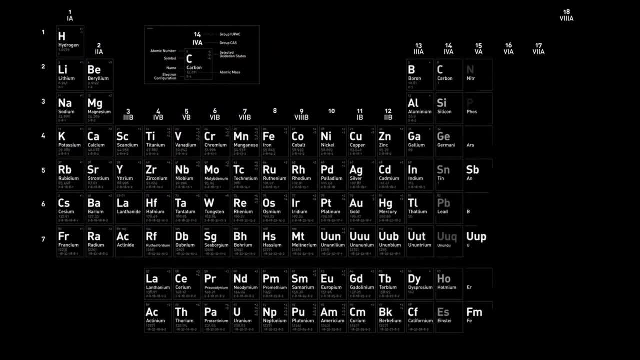 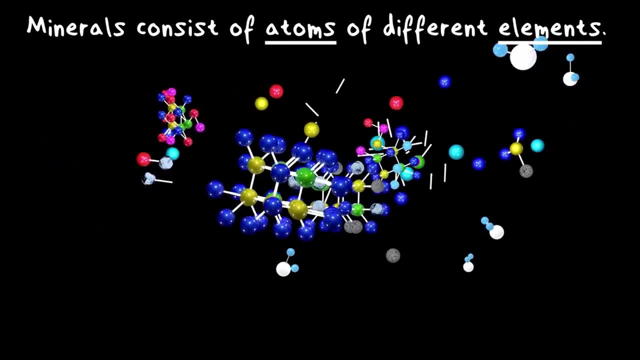 definite chemical composition. All minerals are made out of elements from the periodic table, so there are atoms of these elements that make up the minerals. Minerals are the building blocks of rocks and atoms are the building blocks of minerals. Every single time a mineral exists it has to have. 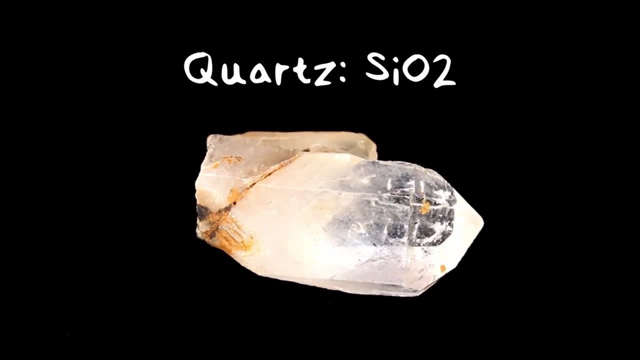 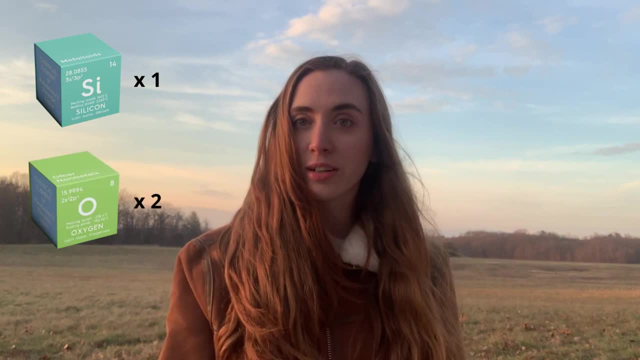 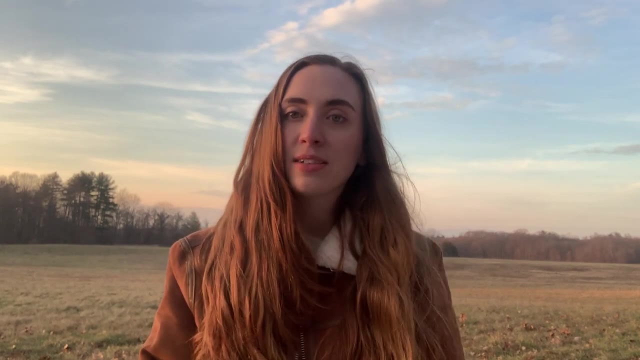 the same proportions of elements. The chemical formula of quartz is SiO2.. This means that there are atoms of silicon for every two atoms of oxygen. I think a good way of thinking about this would be thinking about a family recipe. You try to follow a family recipe the same time, every single time. 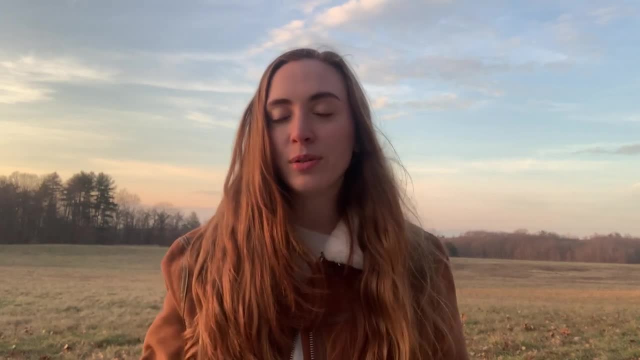 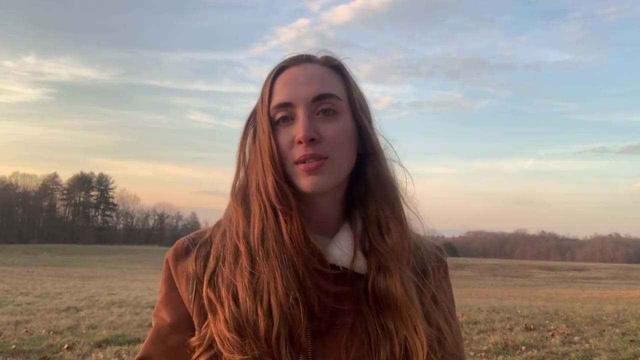 you make it so that it ends up the same thing every single time. So if you took your grandma's chocolate chip cookie recipe and you said I'm gonna put two cups of sugar instead of two cups of flour, it's probably gonna be a very different cookie. The ratios of that cookie recipe are: 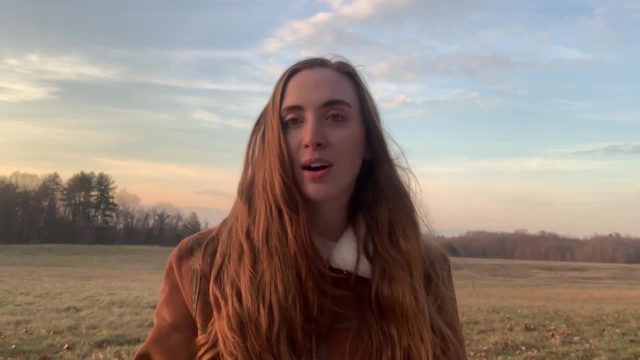 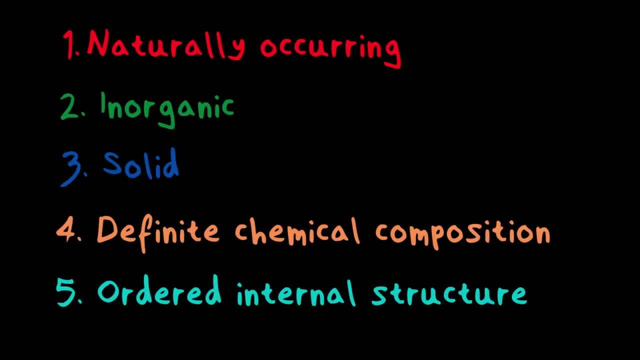 always the same every single time you make it, because you're gonna have the same product every time, the same product that your grandma had. The fifth and last characteristic of all minerals is that they have to have a definite internal structure. So if I took two oxygen atoms and one silicon atom, I can arrange these in a couple. 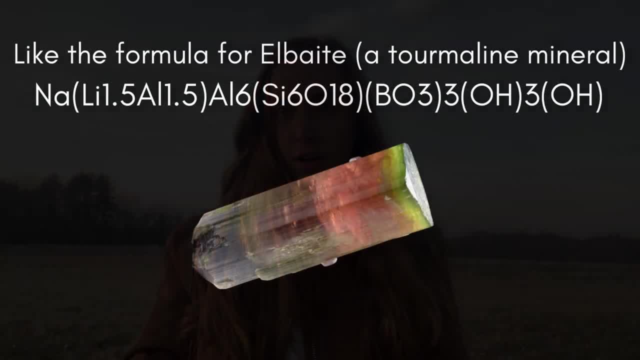 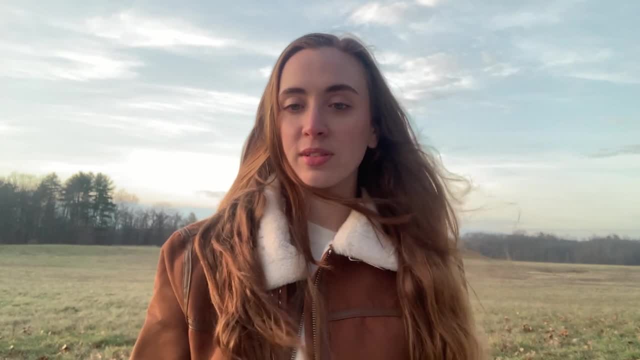 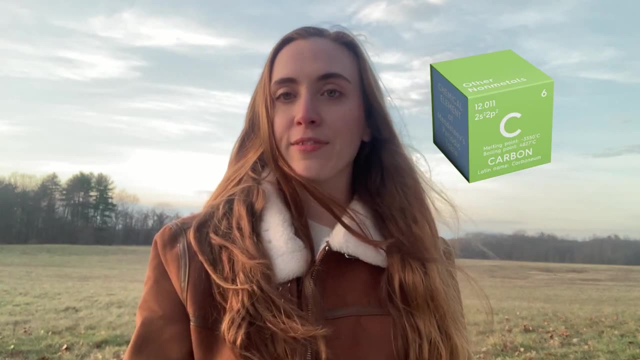 different ways, and this becomes more complicated with the more atoms that there are in that mineral. So because of all these possibilities of the ways that atoms can arrange themselves, we have things like graphite and diamond. They are made of the same element, carbon, but they have very different arrangements of those carbon atoms that make